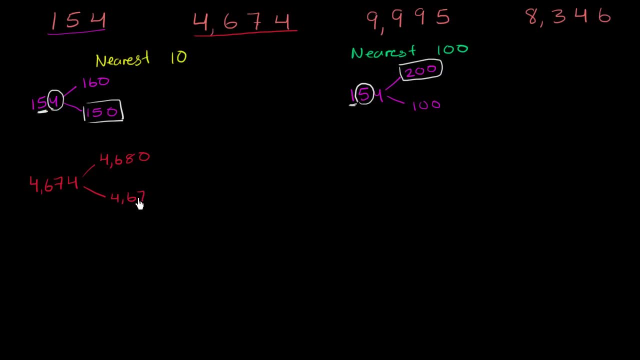 The multiple of 10, below that, 4,670.. Remember, we're concerned only with the multiple of 10.. So do we round up or down? Well, we're thinking about rounding the tens place. So that's why it's either gonna be an eight if we round up. 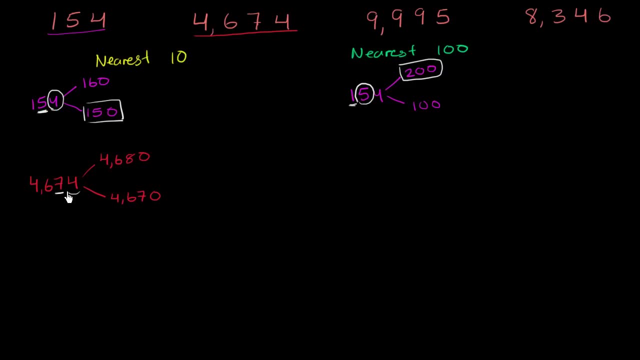 or seven if we round down. To figure that out, we look at the ones place. If the ones place is five or greater, we round up. If it's less than five, we round down. It's once again less than five. so we round down to 4,670. 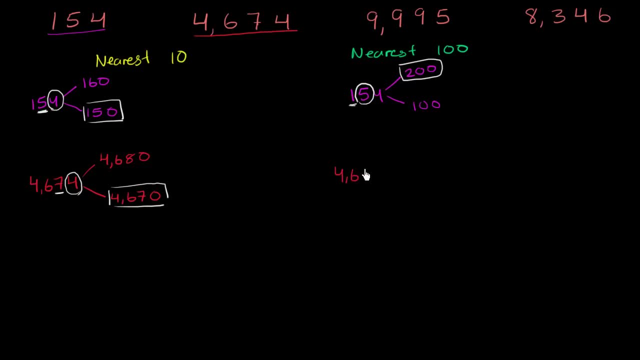 Now let's round the same number to the nearest hundred: 4,674.. What's the multiple of 100 below this? Well, the multiple of 100 below this is 4,600.. The multiple of 100 above this is 4,700. If we're trying to think about rounding to the nearest hundred, Well, the multiple of 100 below this is 4,600.. If we're trying to think about rounding to the nearest hundred, If we're trying to think about rounding to the nearest hundred, 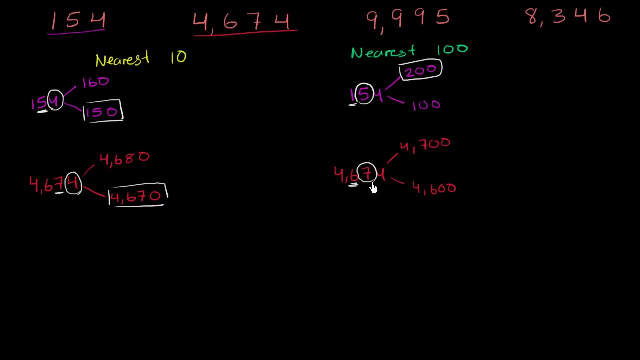 we wanna look at the tens place. The tens place is five or greater, so we round up to 4,700.. Now let's tackle 9,995.. And, once again, always try to pause these if you haven't done so already. 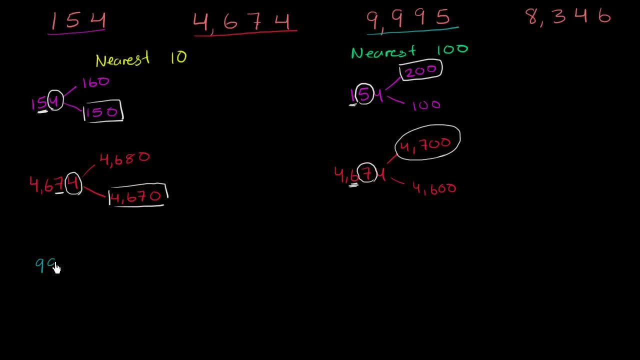 to try to do this on your own, So 9,995.. What is the multiple of 10 below this? Well, the multiple of 10 below this is 9,990.. Well, the multiple of 10 below this is 9,990.. 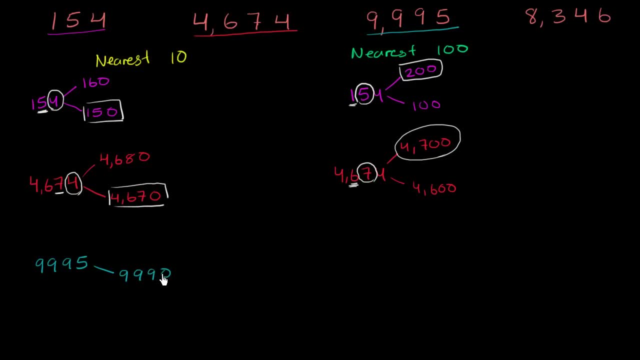 And what's the multiple of 10 above this? Well, if you increase this by 10, you actually get to 10,000.. You get to 10,000.. So you might say, hey, well, isn't this a multiple of 100?? 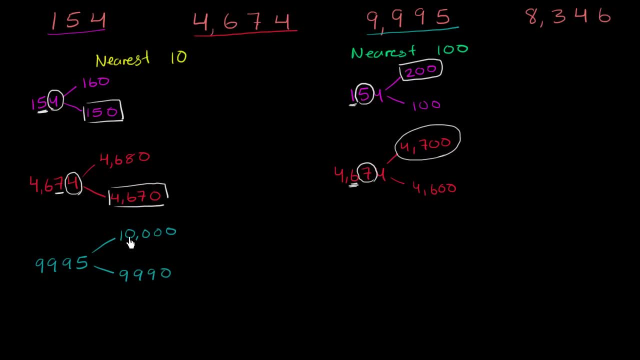 And actually this is a multiple of 1,000. It's also a multiple of 10,000. It's all of those, But the multiple of 10 right above 9,995 is 10,000.. You just have to add a little bit to this to get to 10,000. 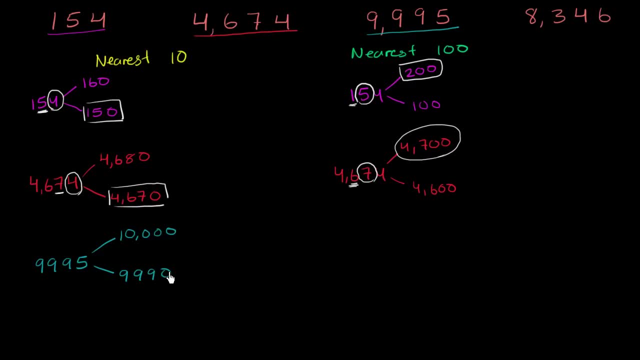 Or the multiple of 10 below it is clearly 9,990.. Ten more than that gets you to 10,995.. Ten more than that gets you to 10,995.. gets you to 10,000.. So how do we round this? 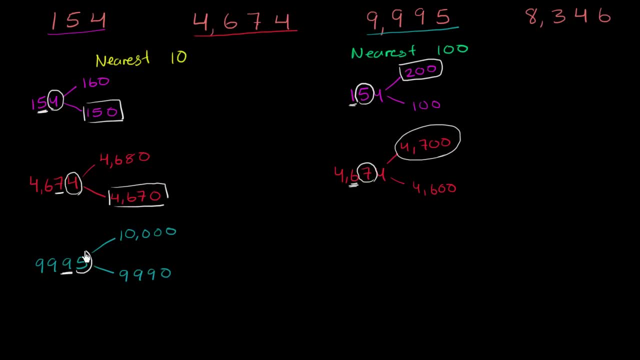 Well, once again, if we're rounding to the nearest 10,, we want to look at the ones place. The ones place is 5 or greater, so we round up to 10,000.. Now let's round to the nearest hundreds. 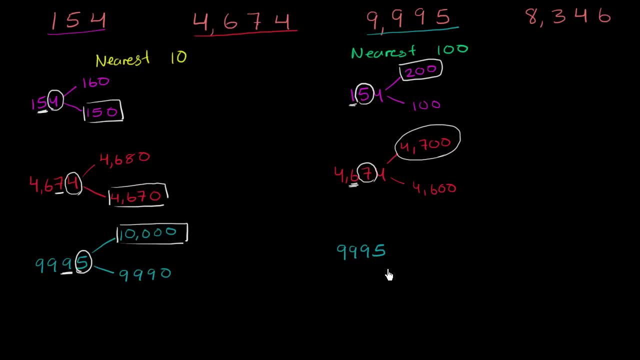 We should be getting used to this. now To the nearest hundreds. What is the hundreds below this? Well, it's 9,900.. What is the hundred above this? What is the next multiple of 100 above this? Well, if you add 100 to 9,900, you once again get 10,000. 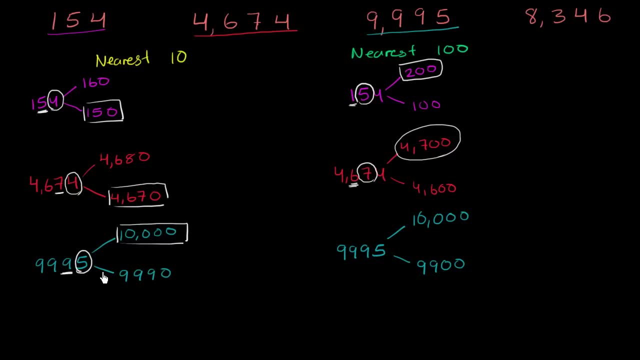 So how do we decide whether to round up or down? Well, we don't look at the ones place anymore. We're now rounding to the nearest hundreds. So we want to round to the nearest hundred. To do that, we look one place to the right. 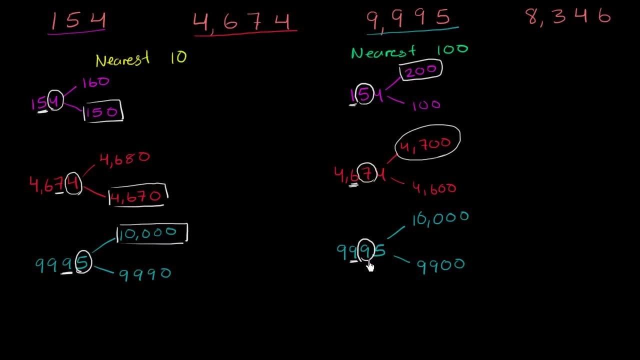 which is the tens place. If this is 5 or greater, we round up. If it's less than 5, we round down. It is 5 or greater. so once again, we round up to 10,000.. Now we have. 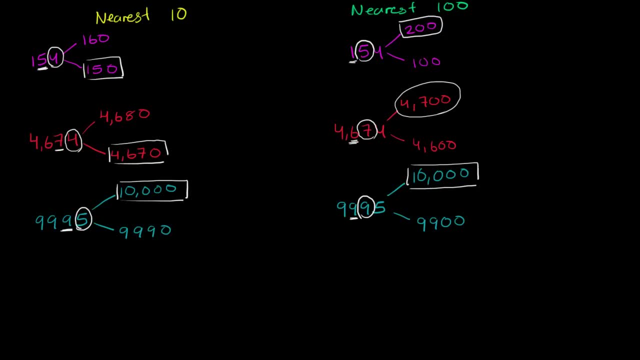 We have one more, 8,346.. So 8,346.. The tens place or the multiple of 10 below it is 8,340.. Multiple of 10 above that is 8,350.. If we're going to round to the nearest 10,. 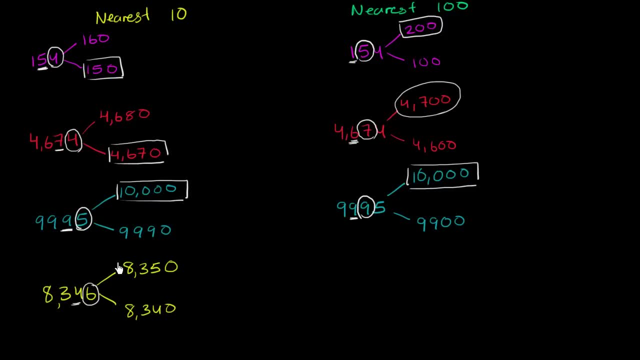 we need to look at the ones place. The ones place is 5 or greater, so we round Up. Now let's round to the nearest hundred: 8,346.. The multiple of 100 above this is 8,400.. 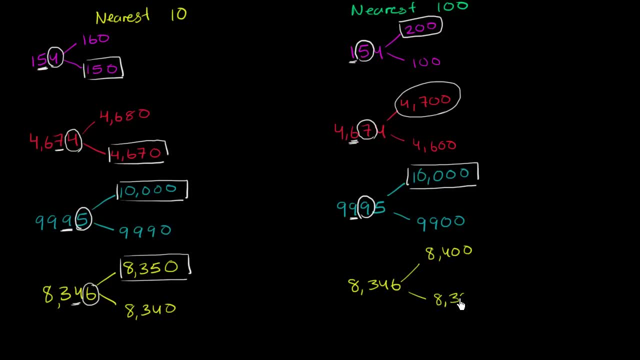 The multiple of 100 below this is 8,300.. Notice, we're rounding to the nearest hundreds. If we were to round up the hundreds, place becomes a 4.. If we were to round down the hundreds, place stays at 3,. 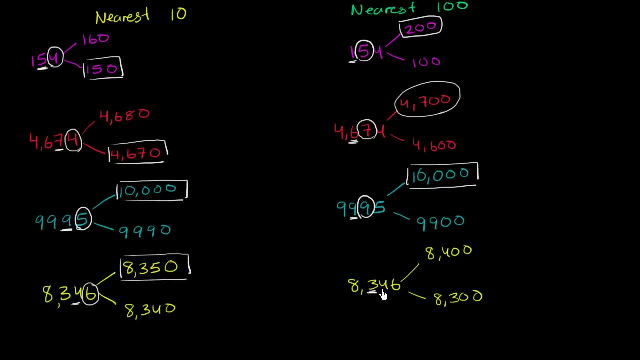 but it's followed by 0's. If we want to round to the nearest hundreds, we need to look at the tens place. The tens place here is less than 5, so we round down to 8,300.. Notice again, when we rounded to the nearest tens. 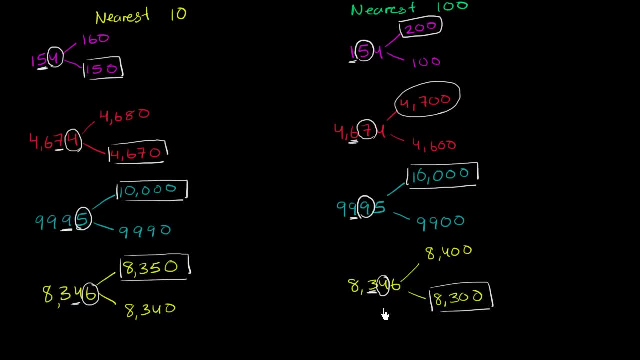 we rounded up to 8,350.. When we rounded to the nearest hundreds, we rounded down to 8,300..